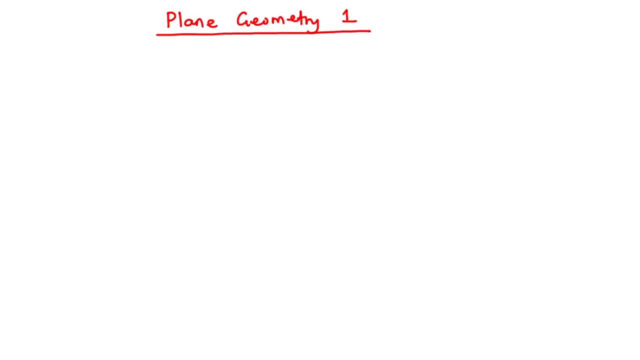 of angles that we have and in the next video we are going to solve a lot of examples on how to calculate or find these angles. So, without wasting much time, let's get into today's video. So angles are formed when two straight lines meet. So, assuming that we have a straight line, 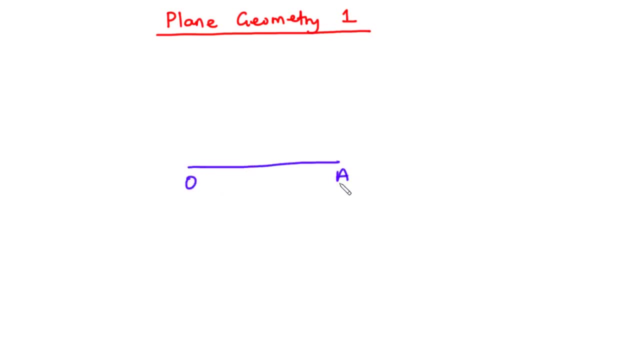 that is OA, and then we also have another straight line, OB. Now, at the point of intersection of these two lines, or at the point where these two lines meet, an angle is formed, And the size of the angle formed can be determined by rotating the line OB. 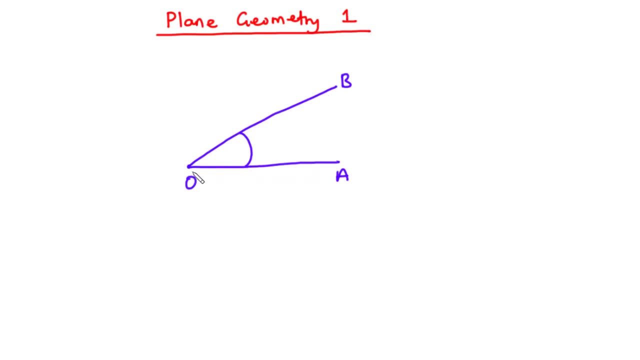 about O in the clockwise direction, to lie on the line OA. Usually, angles are measured with an instrument called a protractor, and I believe that we all know what a protractor is. Now let's move on and talk about the various types of angles that we have. 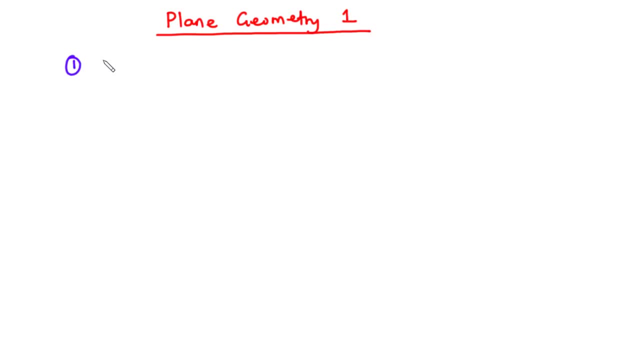 So the first angle we are going to talk about is the angle of the protractor. So the first angle we are going to talk about is the angle of the protractor. Now, the first angle we are going to talk about is what we call the acute angle. 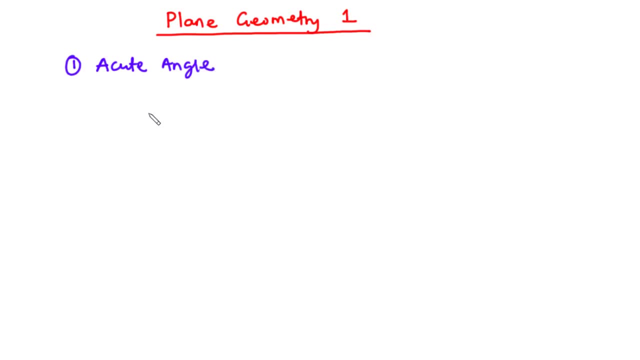 An acute angle is an angle whose measure or size is less than 90 degrees. So, assuming that we have the line OA and then OB, Now the angle formed between these two lines is an acute angle, because this angle is less than 90 degrees. so we say that the angle- this is the symbol. 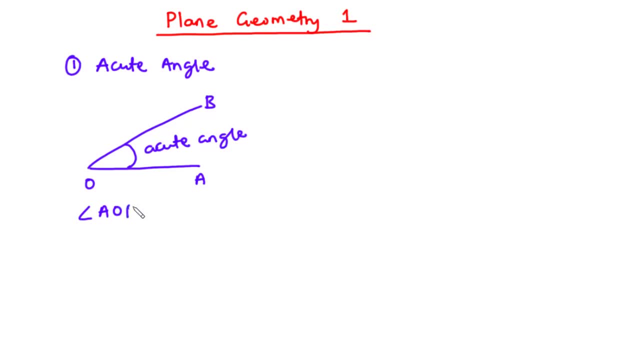 for angle. so the angle a OB, which is this angle, is less than 90 degrees. notice that the two symbols are not the same. this is an angle and then this is the less than sign. so the next type of angle we are going to talk about is the. 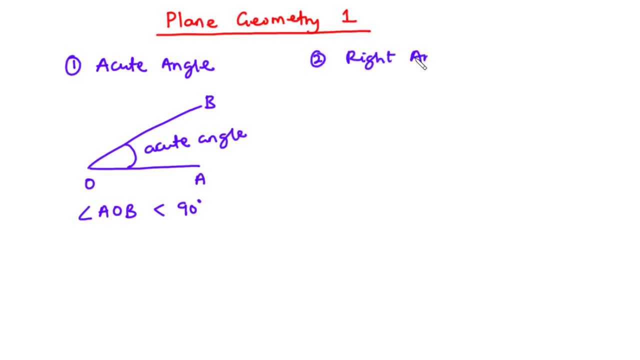 right angle. a right angle is an angle whose measure or whose size is equal to 90 degrees, an angle whose measure or size is equal to 90 degrees. so, as you may have the line OC and then OD, then this angle is the right angle, because that is the angle. 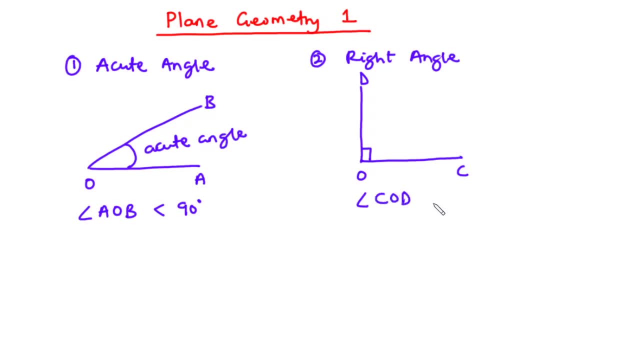 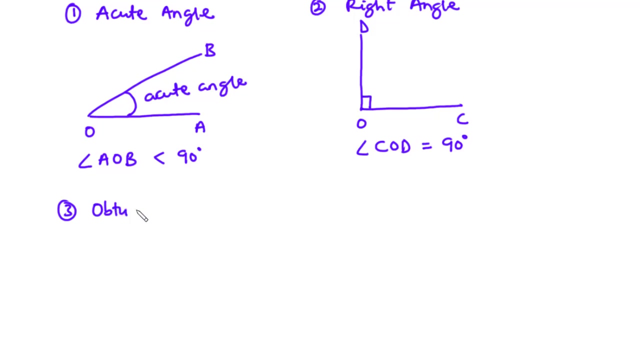 C OD. so angle C OD is a right angle because its measure or size is equal to 90 degrees. now let's move on to the third angle, which is the obtuse angle. the obtuse angle. now for the obtuse angle. it is an angle whose measure or 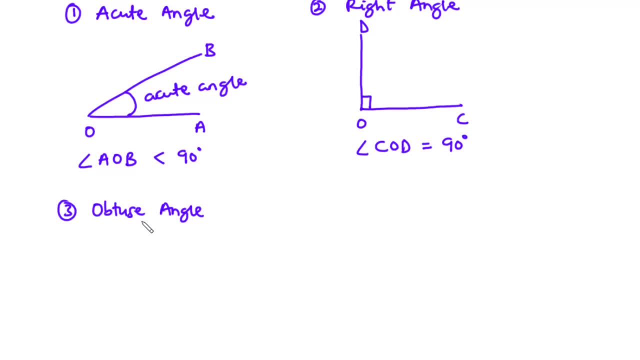 whose size is greater than 90 degrees, but less than 180 degrees. so now let's focus on the right angle. now this angle, but less than 180 degrees. so now let's focus on the right angle. now this angle is 90 degrees, so for this angle we are going. 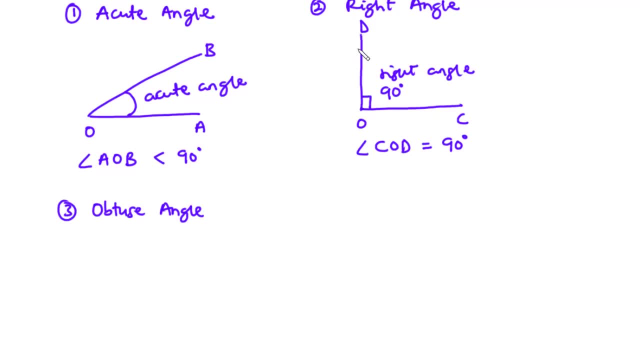 to pull down this line, that is the line OD, in this direction, that is, the anti-clockwise direction, such that it will not lie straight as the line OC. now, in that case, the new angle formed is greater than 90 degrees, but less than 180 degrees. so for obtuse angle to the left of oxido line, we're going to pull. 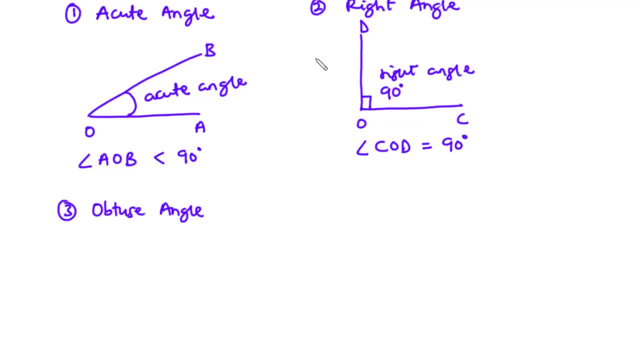 another line back down and once again let's talk about behavior- is e zero and is greater than 90 degrees but less than 180 degrees. So assuming this is the line OE, and then we have another line OF. Now this is an obtuse angle because the angle formed, that is the angle EOF, is greater. 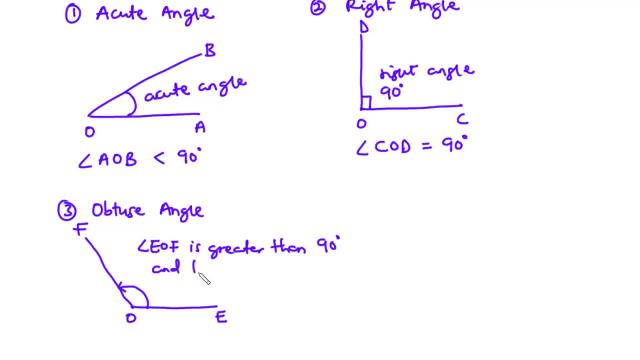 than 90 degrees and less than 180 degrees. So this angle is an obtuse angle. Okay, Now to the next one. So the next one we are going to talk about is the straight angle, The straight angle. Now, the straight angle is an angle whose measure or size is equal to 180 degrees. 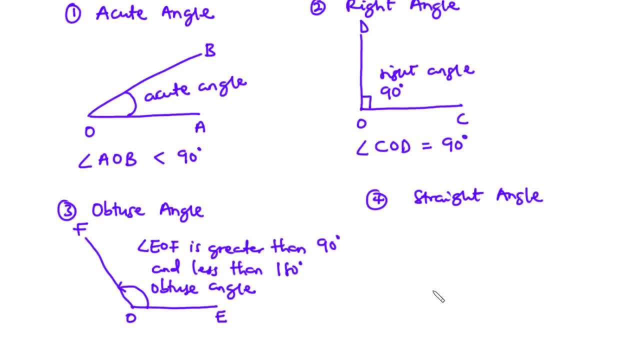 Basically we say that the angle formed on a straight line is equal to 180 degrees. So the angle that is angle MON is a straight angle. So that angle that is angle MON, is a straight angle And it's equal to 180 degrees. 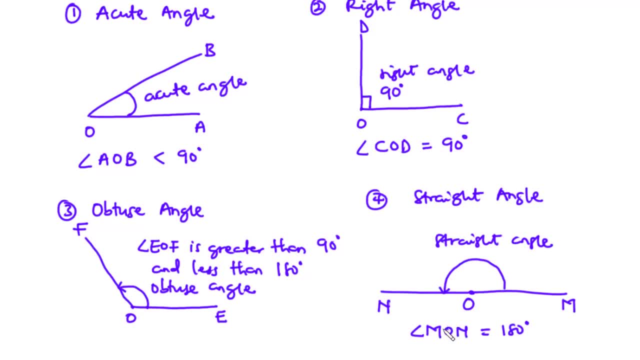 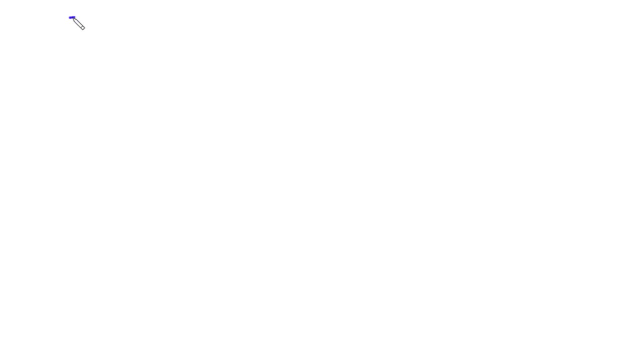 So the next type of angle which we talk about for straight line is calleditions, And to do that, The we are going to talk about is the reflex angle. The reflex angle is an angle whose measure or size is greater than 180 degrees but less than 360 degrees. So let's consider the angle, assuming 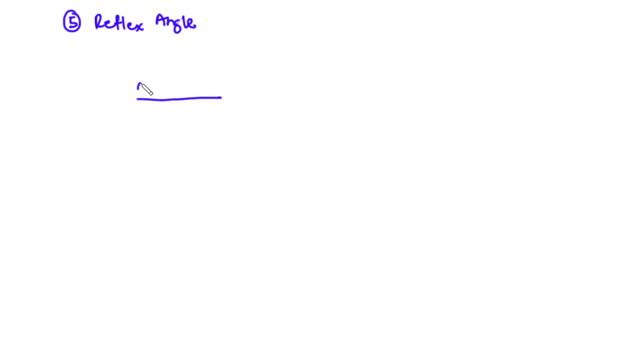 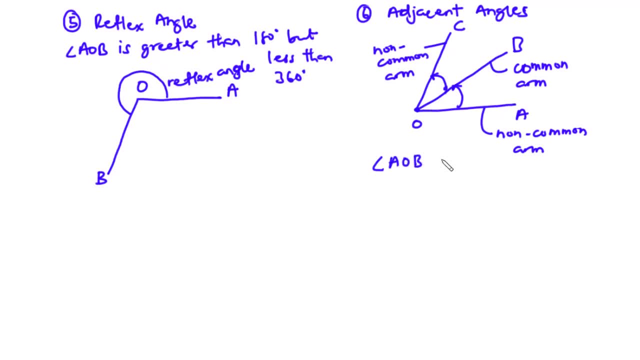 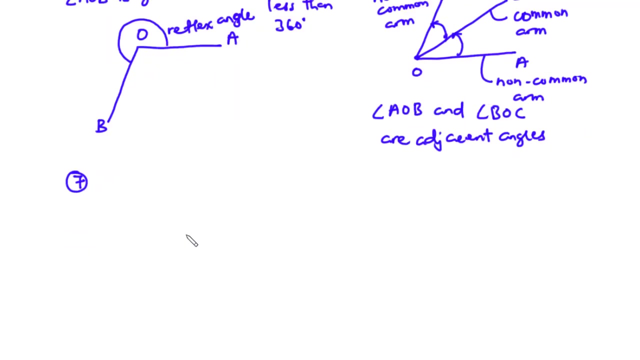 OB and then B OC. they are adjacent angles. okay, so now let's move on to the next type of angle, that is what you call complementary angles. so complementary angles are two angles that add up to 90 degrees. so let's consider the right angle. so the right angle has a measure. 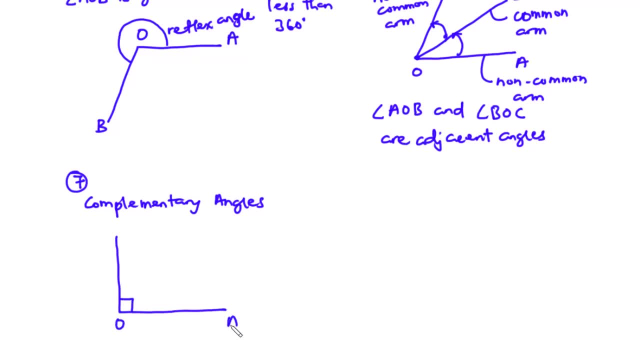 of 90 degrees. so, assuming this is OE and this is OB, and then we have the line OC. now here we have two angles formed and these two angles sum up to 90 degrees. so we say that the angles AOC and B OC are complementary angles. 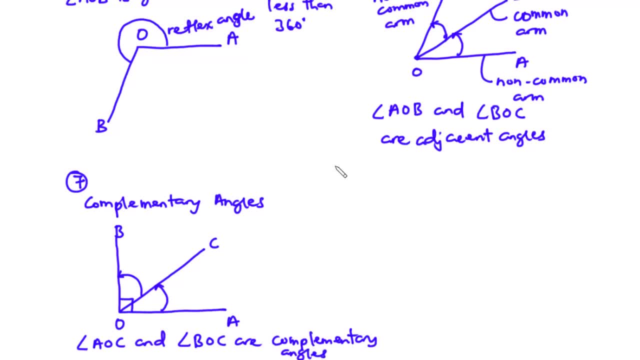 now to the next one. we call that supplementary angles. so supplementary angles are two angles that add up to 180 degrees. so let's consider the straight angle. the angle on a straight line is 180 degrees. so if we have two angles adding up to 180 degrees, then they are. 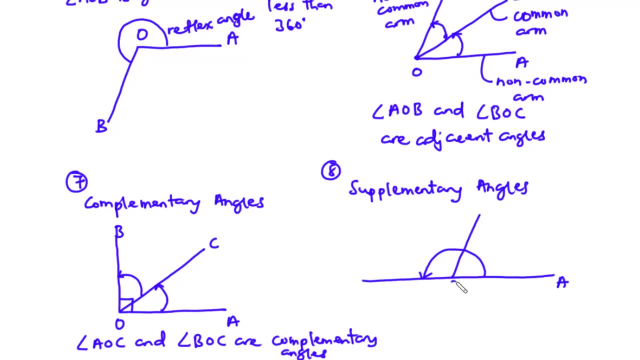 supplementary angles. therefore we say that the angles AOB and BOC are supplementary angles. so angle AOB plus angle BOC is equal to 1, 80 degrees, and here also the angles AOC plus BOC is equal to 90 degrees. now let's move on to the type of angle we are using here. 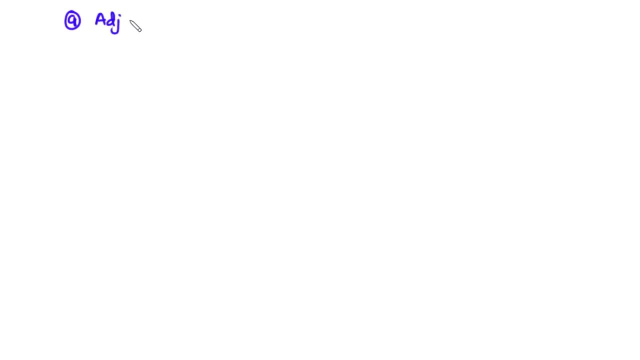 angles we call adjacent supplementary angles adjacent supplementary angles. now, these angles are basically like the adjacent angles and for these type of angles, assuming that we have a straight angle angle, now we have two angles adding up to 180 degrees. so this is o a, o b and then o c. 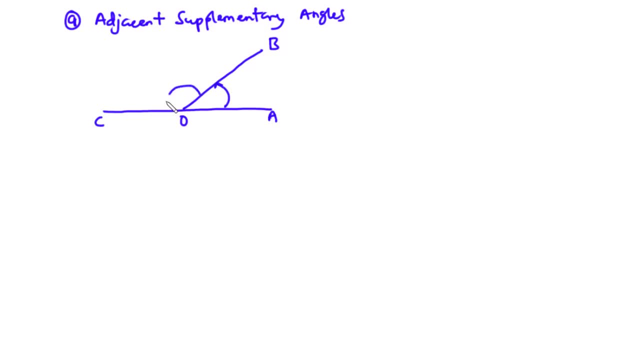 now, because they are adjacent supplementary angles. we have this to be the common arm and then o e and then o c are the non-common arms and then they have a common vettus. so we call these adjacent supplementary angles. so the angles a o b plus b o c. they sum up to 180 degrees away from that if we have a straight angle. 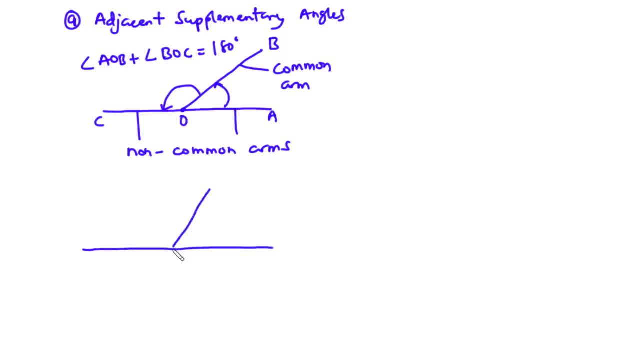 and then we have more than 180 degrees, two angles adding up to 180, assuming that we have angle a, angle b and then angle c. now these three angles- a, b, c- are sub to 180 degrees. now let's move on to angles around a point. 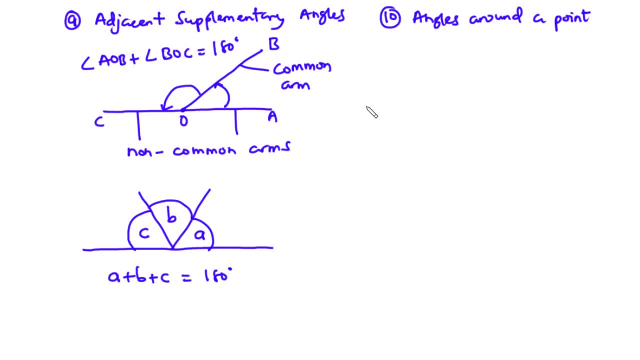 so when many lines meet at a point, they form angles around a point and the sum of these angles are equal to 360 degrees. so, assuming that we have three lines meeting at a point, we have this to be angle x, angle y and then angle z. now the sum of these angles are equal to 360 degrees. 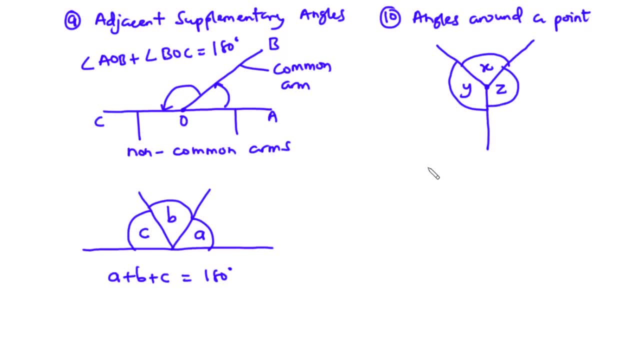 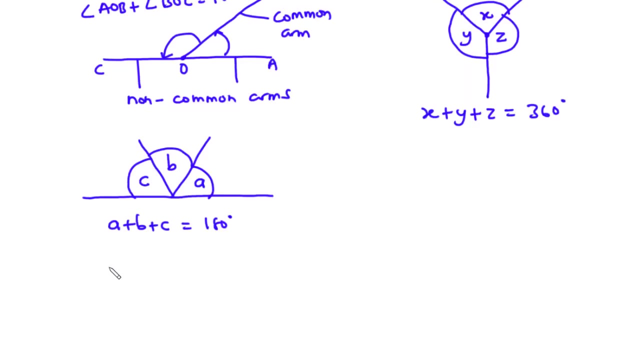 is equal to 360 degrees. So we say that x plus y plus z is equal to 360 degrees. So that is that with angles around a point. Now let's move on to vertically opposite angles. So when two straight lines meet at a point, four angles are formed at the point of intersection. 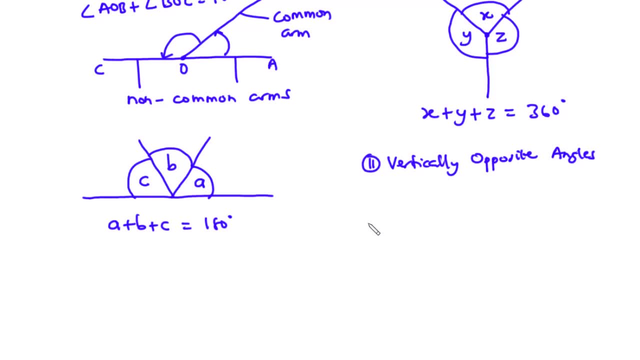 Now the angles on the opposite sides of the point of intersection are called vertically opposite angles. So assuming that we have two lines meeting at a point, This is the point of intersection. Let's say the angle here is A, the angle here is B, the angle. 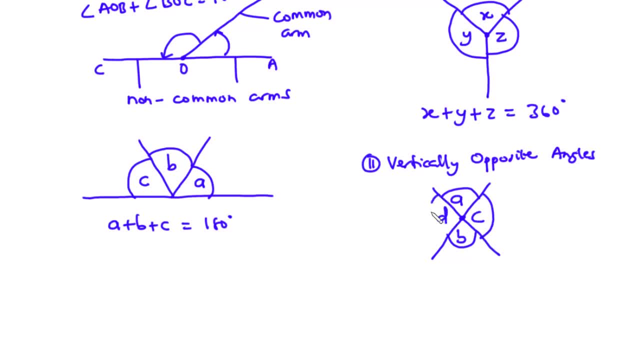 here is C, And then also we have angle D here. So we are saying that when two straight lines meet at a point, four angles are formed at the point of intersection, And the angles on the opposite sides of the point of intersection are called vertically opposite angles, and they are equal. 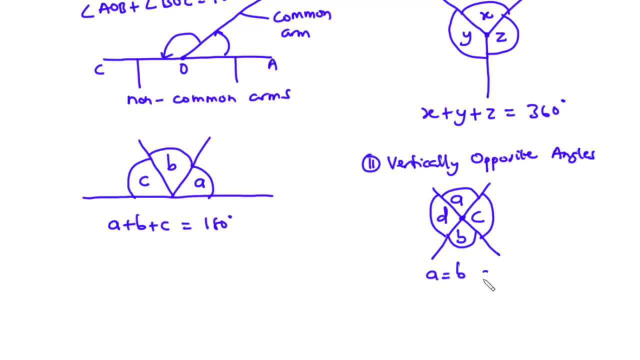 So angle A is equal to angle B and angle C is equal to angle D. So we say that angle A and B are vertically opposite angles, And then C and D are also vertically opposite angles. Now to the last one. let's talk about perpendicular lines. 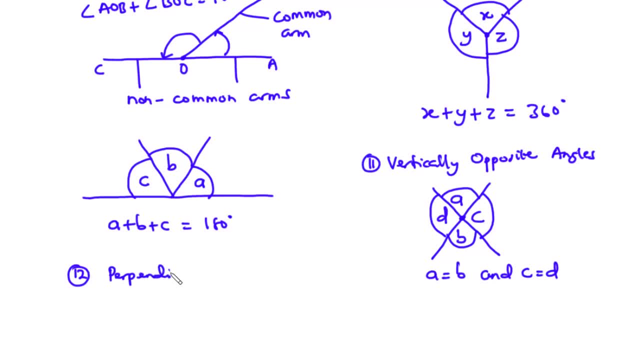 Two lines are said to be perpendicular if they meet or intersect at right angles. So when two perpendicular lines meet, four right angles are formed. So, assuming that we have two perpendicular lines, we have two right angles. So we have two right angles. 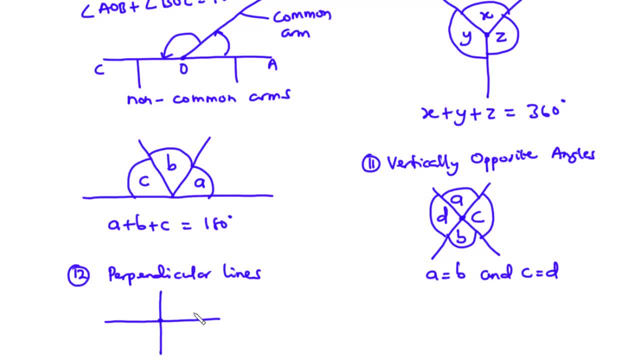 We have two perpendicular lines And this is the point of intersection of these two lines. So we have OA, OB, OC and then OD. So at the point of intersection four right angles are formed. So we say that the line AC is perpendicular to the line BD. 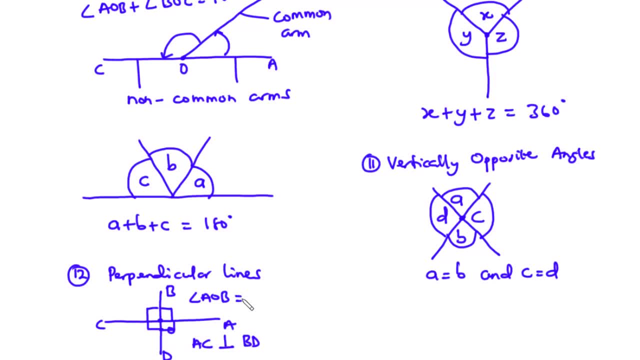